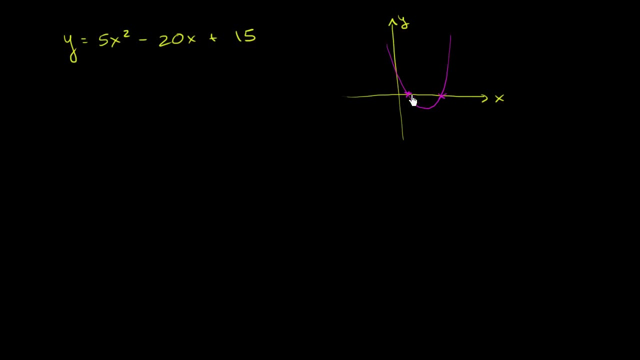 intersect the x-axis And, as we've already seen, intersecting the x-axis is the same thing as saying: when does y equal 0? For this parabola, Or another way of saying it: when does this? 5x squared minus 20x plus 15,? when does this? 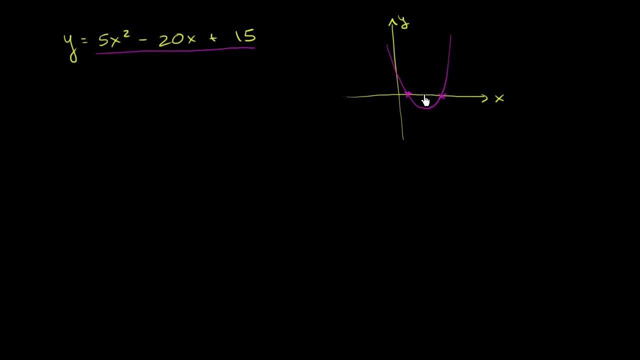 equal 0?. So I want to figure out those points, And then I also want to figure out the point exactly in between, which is the vertex. And if I can graph those three points, then I should be all set with graphing this parabola. 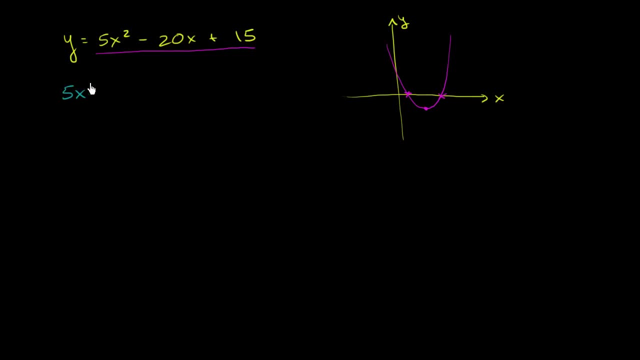 So, as I just said, we're going to try to solve the equation: 5x squared minus 20x plus 15 is equal to 0.. Now the first thing I like to do whenever I see a coefficient out here on the x squared term, that's not a 1. 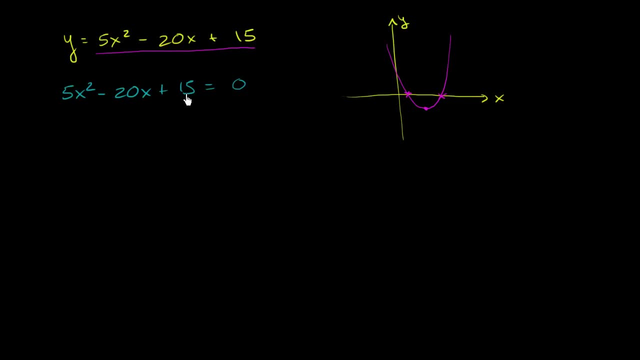 is to see if I can divide everything by that term to try to simplify this a little bit And maybe this will get us into a factorable form. And it does look like every term here is divisible by 5. So I will divide by 5.. 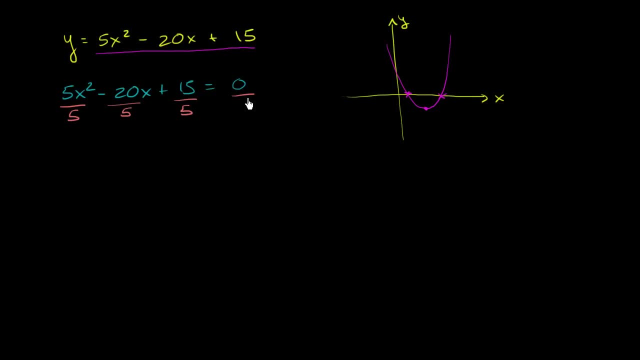 So I'll divide both sides of this equation by 5.. And so that will give me these: cancel out and I am left with x squared: minus 20 over 5 is 4x. plus 15 over 5 is 3 is equal to 0. over 5 is just 0.. 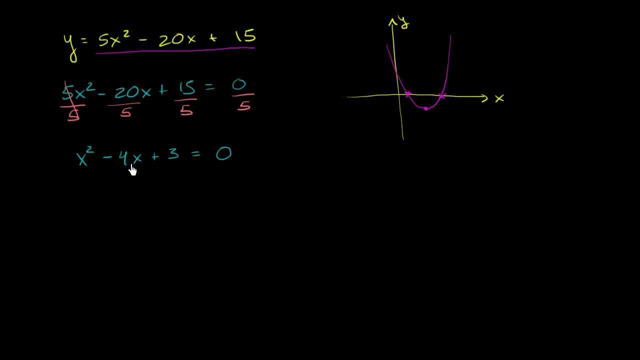 And now we can attempt to factor this left-hand side And we say: are there two numbers whose product is positive? 3, the fact that their product is positive tells you that they both must be positive. and whose sum is negative? 4, which tells you well, 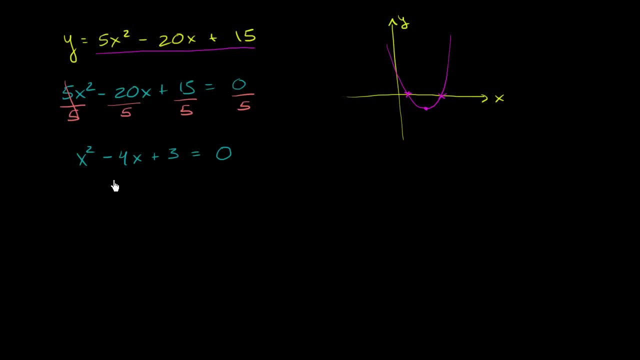 they both must be negative. if we're getting a negative sum here- And the one that probably jumps out at your mind- and you might want to review the videos on factoring quadratics if this is not so fresh- is negative 3 and negative 1 seem to work. 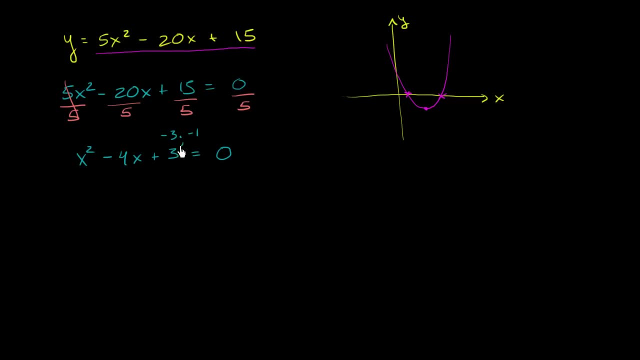 Negative 3 times negative: 1. Negative 3 times negative: 1 is 3.. Negative 3 plus negative 1 is negative 4.. So this will factor out as x minus 3 times x minus 1.. And on the right-hand side we still have that being equal to 0.. 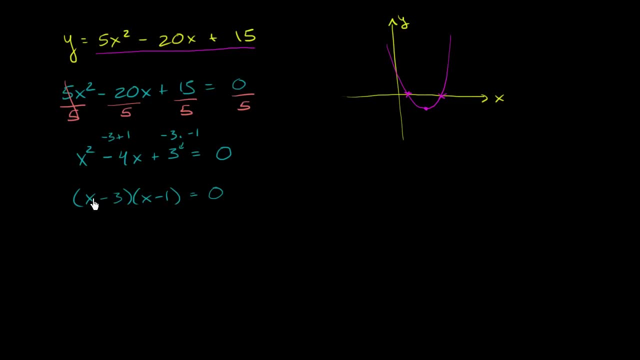 And now we can think about what x's will make this expression 0. And if they make this expression 0,, well, they're going to make this expression 0,, which is going to make this expression equal to 0. And so we're going to do that. 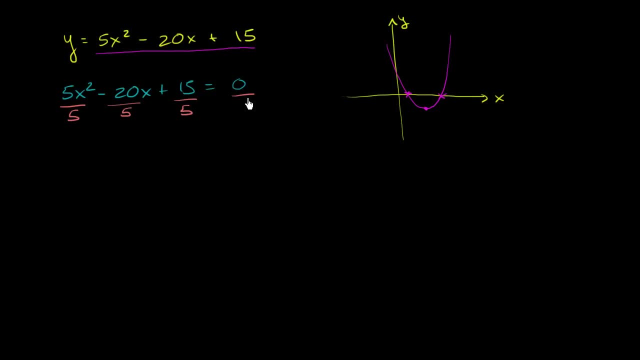 So I'll divide both sides of this equation by 5.. And so that will give me these: cancel out and I am left with x squared: minus 20 over 5 is 4x. plus 15 over 5 is 3 is equal to 0. over 5 is just 0.. 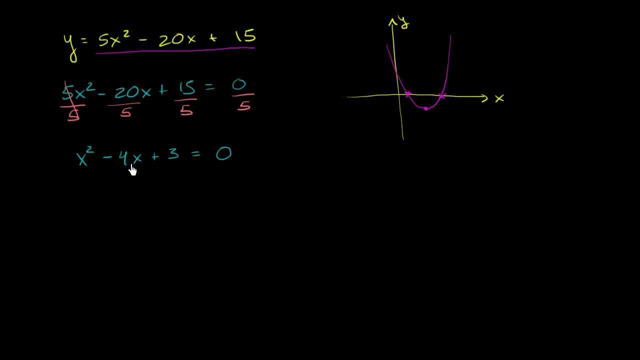 And now we can attempt to factor this left-hand side And we say: are there two numbers whose product is positive? 3, the fact that their product is positive tells you that they both must be positive. and whose sum is negative? 4, which tells you well, 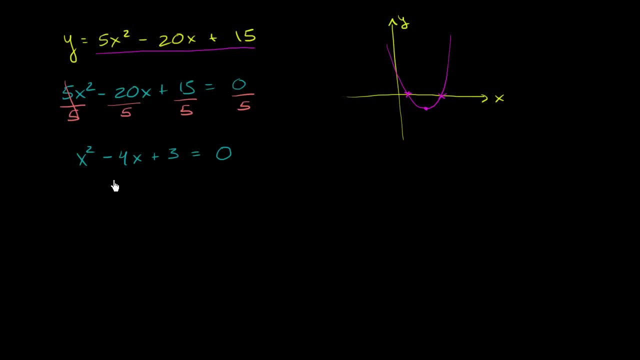 they both must be negative. if we're getting a negative sum here- And the one that probably jumps out at your mind- and you might want to review the videos on factoring quadratics if this is not so fresh- is negative 3 and negative 1 seem to work. 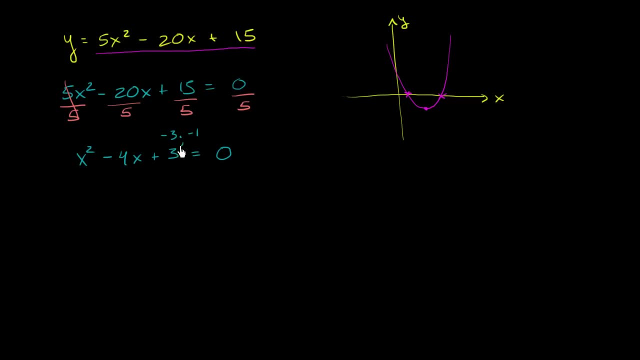 Negative 3 times negative: 1. Negative 3 times negative: 1 is 3.. Negative 3 plus negative 1 is negative 4.. So this will factor out as x minus 3 times x minus 1.. And on the right-hand side we still have that being equal to 0.. 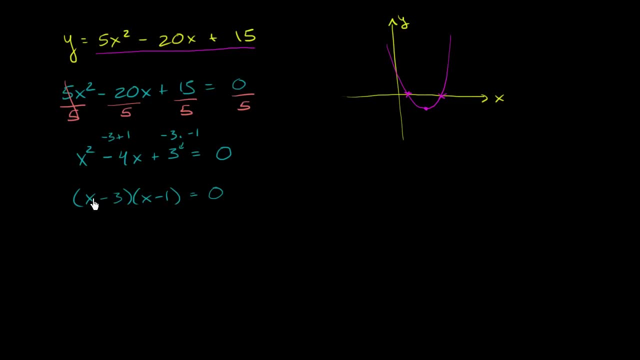 And now we can think about what x's will make this expression 0. And if they make this expression 0,, well, they're going to make this expression 0,, which is going to make this expression equal to 0. And so we're going to do that. 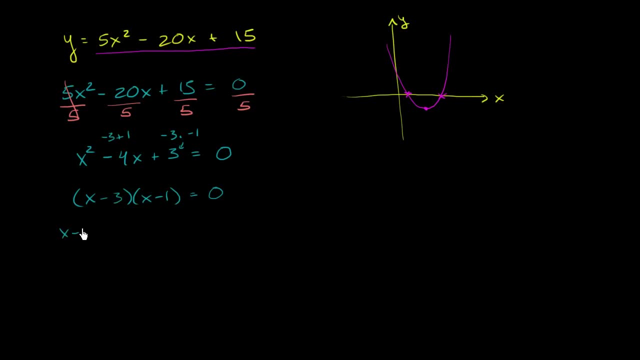 And so this will be true if either one of these is 0. So x minus 3 is equal to 0, or x minus 1 is equal to 0. This is true, and you can add 3 to both sides of this. 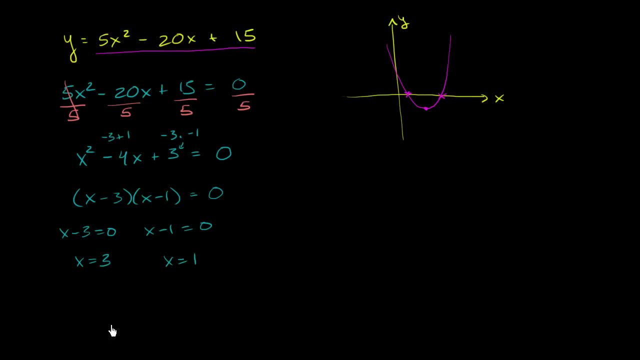 This is true when x is equal to 3.. This is true when x is equal to 1.. So we were able to figure out these two points right over here. This is x is equal to 1.. This is x is equal to 3.. 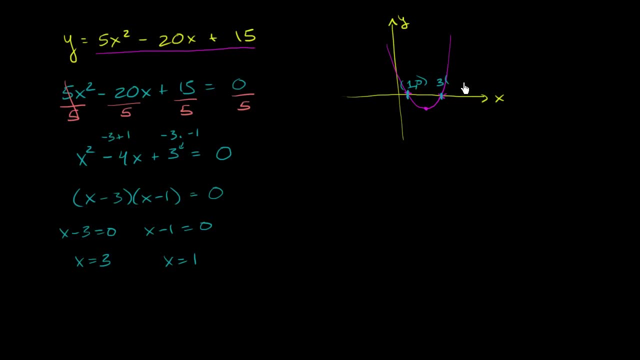 So this is the point 1 comma 0.. This is the point 3 comma 0.. And so the last one I want to figure out is this point: right over here, The vertex. Now the vertex always sits exactly smack dab between the roots. when you do have roots, 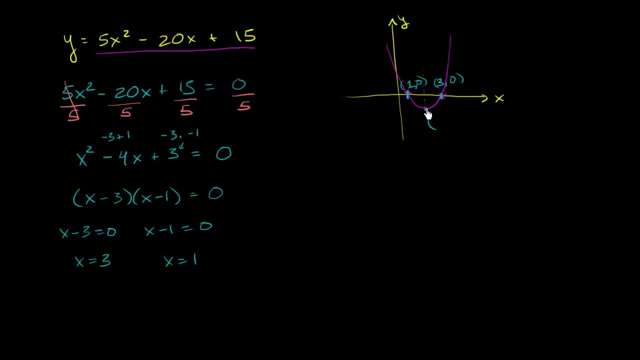 Sometimes you might not intersect the x-axis, So we already know what its x-coordinate is going to be. It's going to be 2.. And now we just have to substitute back in to figure out its y-coordinate. When x equals 2, y is going to be equal to 5 times 2 squared.